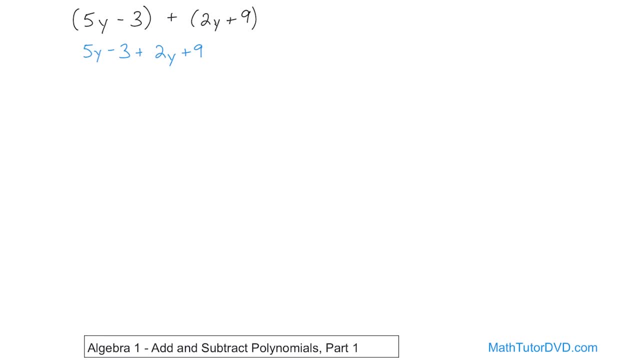 numbers, because they're both talking about the same variable, So we can add them. What is 5 plus 2?? By the way, don't let this subtraction scare you. this or throw you off. This subtraction applies to the 3.. This is a positive 5y. This is a positive 5y. This is a positive 5y. This. 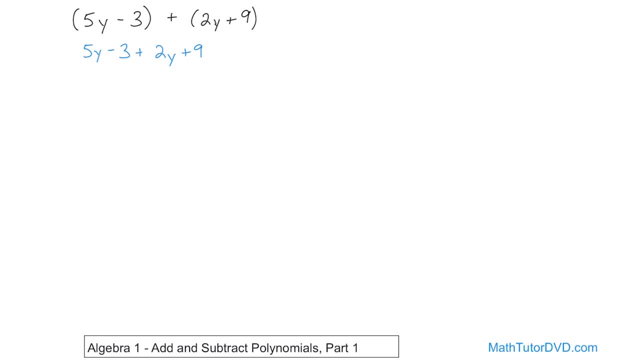 is a positive 2y. So we add them together. normally 5 plus 2 is 7.. So what you're going to get is 7y. Don't forget, the variable has to come along for the ride. It's like 5 jelly. 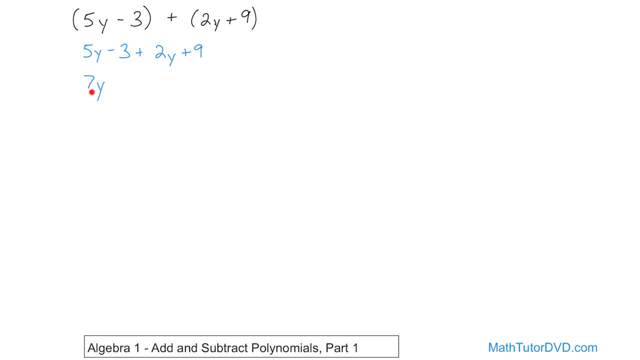 beans and 2 jelly beans. You add them together, you get 7 jelly beans, So the variable comes along for the ride. Then you start looking for other like terms. You have a negative 3 and you have a positive 9.. There's no variable associated with any of those, so those are. 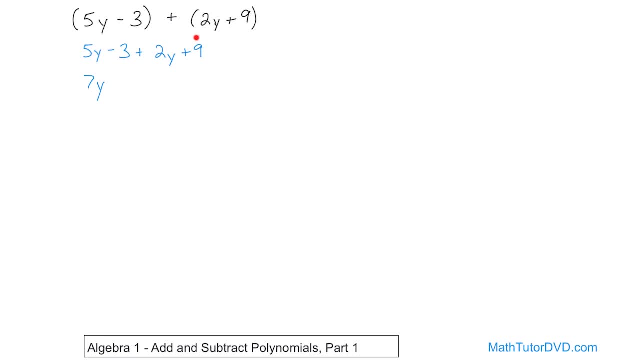 just numbers, So of course you can add them together. What is negative? 3 plus 9?? The way you handle that is by subtracting Subtraction. 9 minus 3 is 6. And the sign goes with the larger absolute value, which. 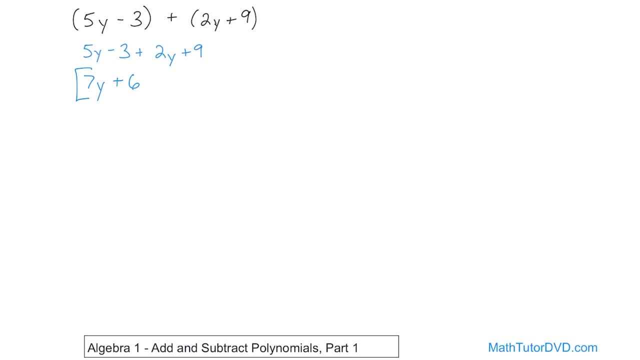 is 9.. So it's going to be a plus sign. So the answer to this is 7y plus 6.. So congratulations. you've added together two polynomials. This is a binomial because it has two terms. This is a binomial because it has two terms And we just added them together. So every problem. 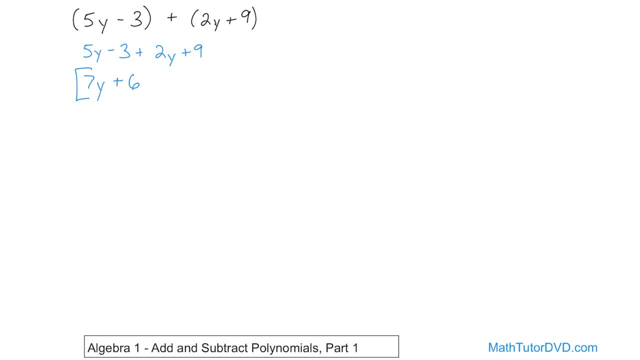 we do is going to be like this: You're going to look for like terms and you're going to add them together, And that's all that there really is to it. So, to take another example, what if we had, for instance, 3x plus 8.. And we're going to add to it 2x minus 5.. Just, 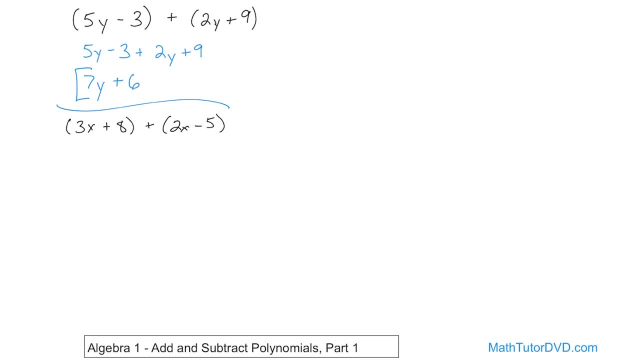 like this. So same sort of thing. So you can mentally drop the parentheses if you want, or you could just write it all out, Just for the first couple times. we'll write it all out. We're able to drop them because there's nothing to do in here. You can't add these. 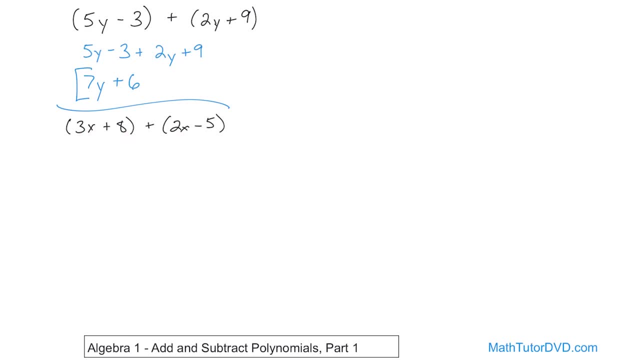 together. They're unlike Same thing there, So you can just kind of write it all down: 3x plus 2x minus 5.. And you don't have to do that, but it sometimes makes it easier to see that you have three x's and two x's. They're both positive, so you can just add. 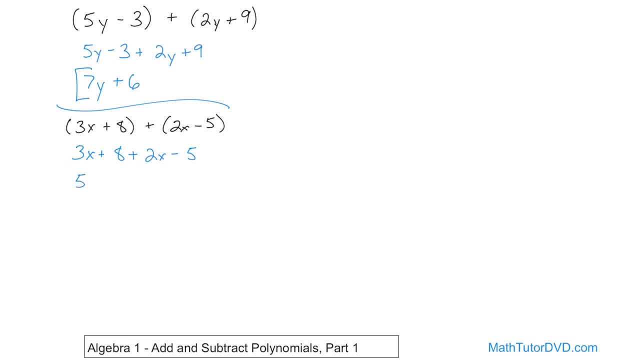 them together because they're like terms: 3 plus 2 is 5, so you get five x's. And then you look you have 8 and you have negative 5.. So how do you add 8 to negative 5?? Or you: 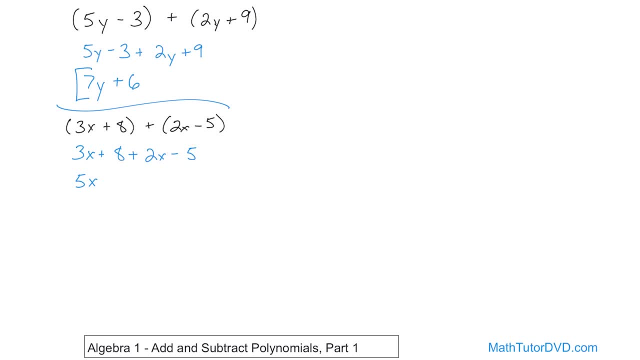 can read it as 8 minus 5.. 8 minus 5 is just simply 3.. So positive 3. And the answer is 5x plus 3.. All right, So it's pretty simple. That's what we're going to be doing. You're always going to be hunting. 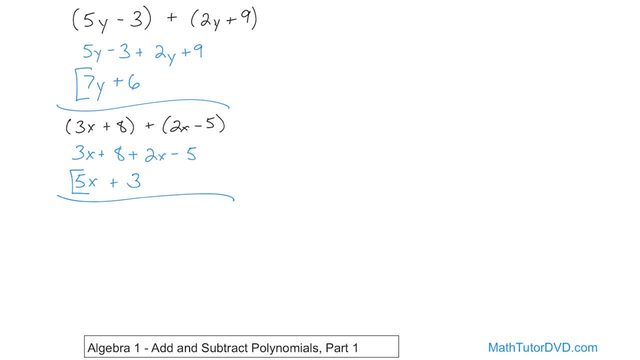 for like terms in order to add them. What if you had- let's take something a little bit bigger- What if you had 2r minus 3x plus 5 plus negative r plus 3x minus 2?? So again, 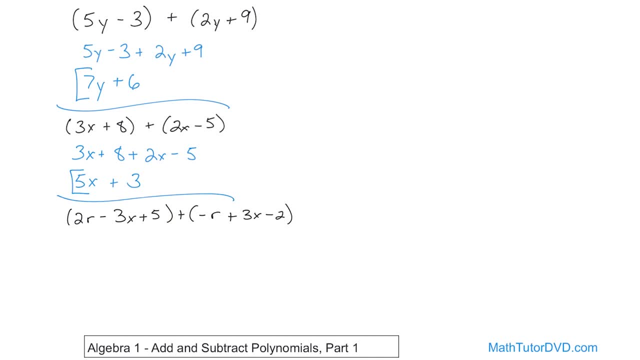 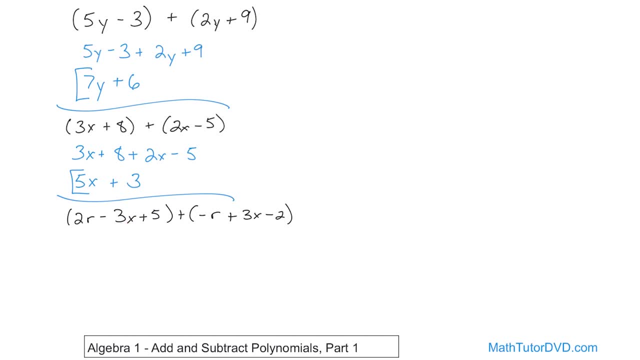 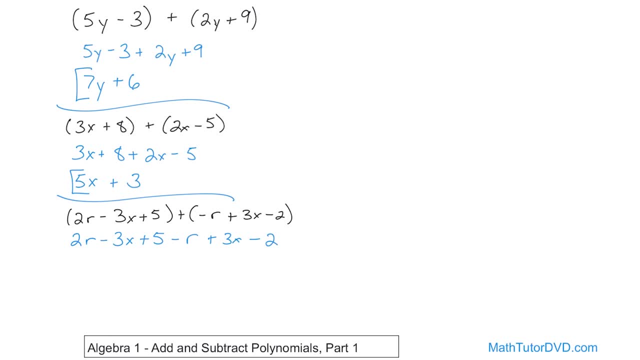 so when you read it like this, just write it as subtraction here and here. basically, the signs are coming from inside of there. so now that we have it all written down, we're start start to hunt for these like terms. so we see that we have two r's, positive two r, and here we have negative r, right. 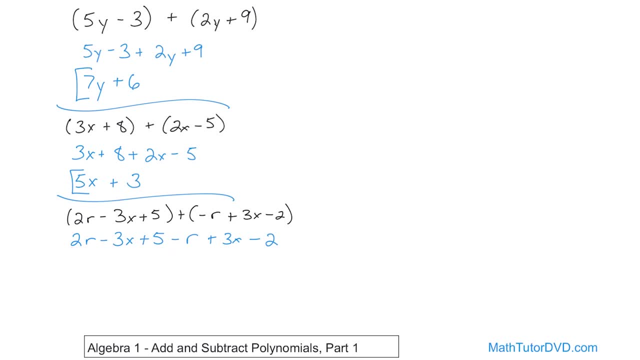 so how do you add those together? you can also read this: two r minus r or two minus one. so that's just going to give you a positive one, or positive r in this case, because you have to keep the variable. so basically, the subtraction of two r minus r just simply becomes r or one r. and what? 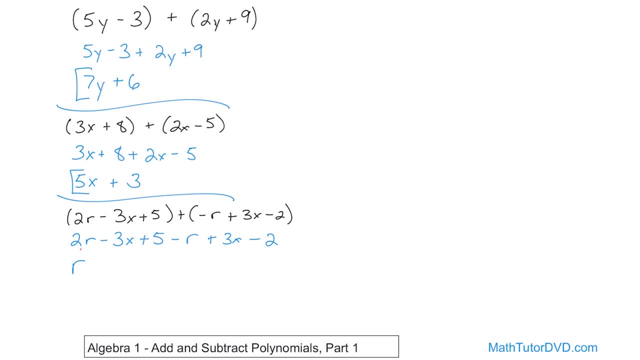 I like to do when you have lots and lots of terms like this is: after I add things together, I put a little dot underneath it and the dot reminds me that I've already handled those two terms. so now I can go and look at other things and look for other things that are similar. so here I have. 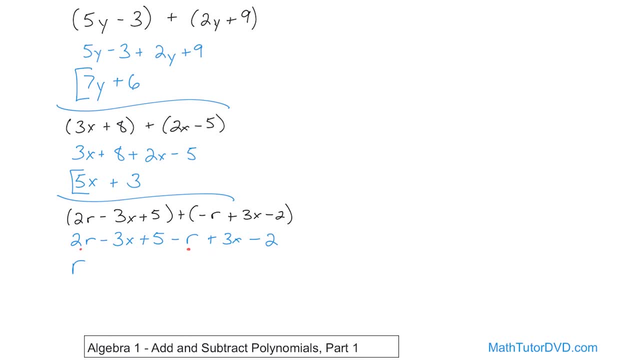 negative three x, and here I have positive three x. what's that going to add together to equal negative three plus three is going to be zero. so instead of writing zero down, I'm just going to strike through this and strike through this. and that reminds me that. 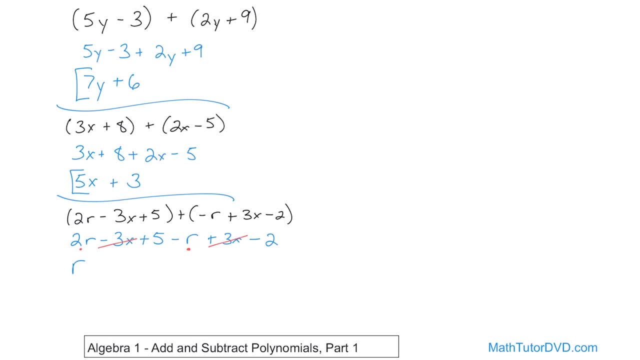 they've. they don't really, I guess, vanish into thin air. it's just that they add together to give you zero, so you don't write anything down for those. and here you have five minus two, or five plus a negative two, if you want to think of it that way, but it's five minus two which is going. 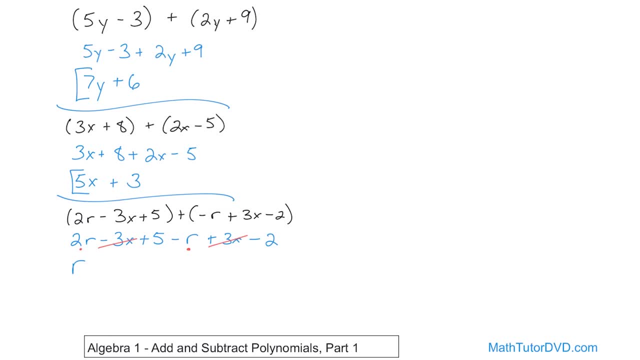 to give you a positive three. so we'll go change the color back here and give us positive three. so the answer is r plus three. that's the final answer. so again, you just write everything down, look for these uh like terms and then go to town trying to trying to simplify them. what if you have? 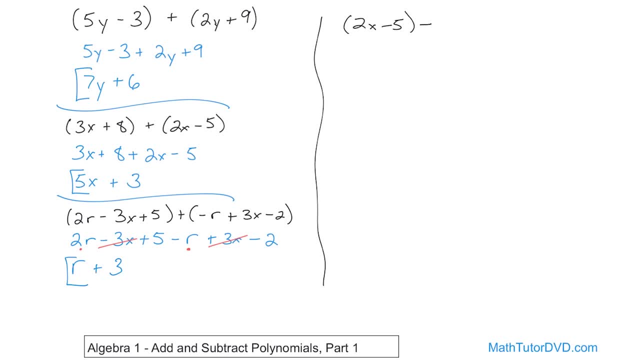 two x minus five minus x minus two. now here's our first problem, where we're subtracting polynomials. you see, here we were adding polynomials together in all three cases. here we have a polynomial- a binomial in this case, and we're subtracting from it another binomial. so here you do have to be. 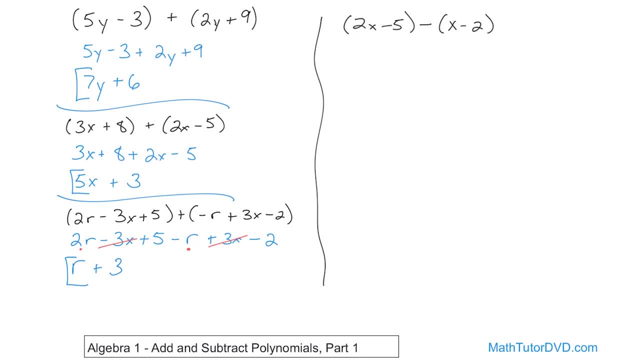 able to do that. so you have this minus sign. so you really do need to write everything down before you try to do the subtraction. so, for instance, you're going to have two x minus five. we can drop those parentheses. but here you see this negative- it's really a negative one out here. you need to. 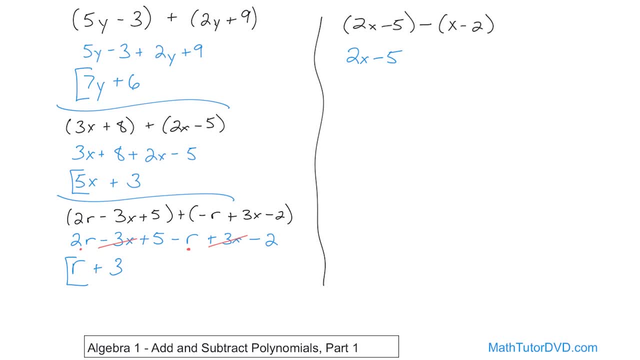 distribute it into here and distribute it into there. remember that distributive property. I told you that you'd be using it over and over again and you will be, so this is going to be written as minus x. let me switch back here. minus x, and what do you think is going to happen when you distribute the 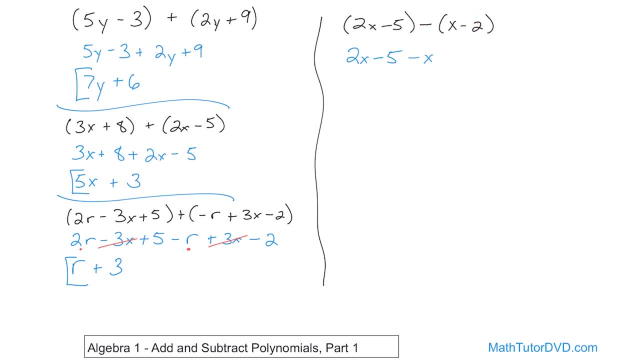 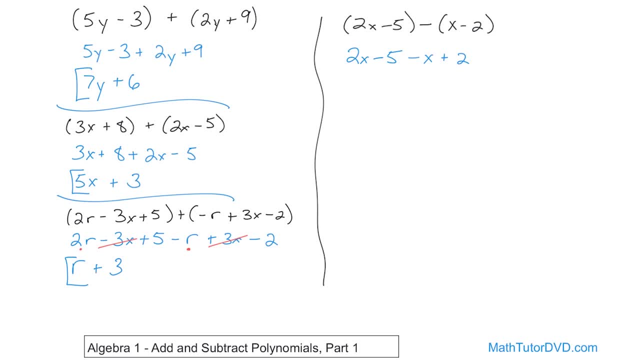 of multiplication in algebra. so now you start looking for like terms. you have positive two x minus x, or you can read it as two minus one, because there's an implied one here. two minus one is one, and of course you still have to keep the x, so it's going to be x. and then you have 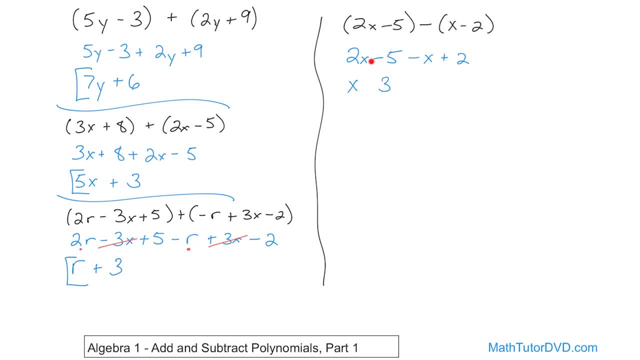 to subtract five minus two is three and the sine goes with the larger absolute value which is negative five. so it's going to be x minus three and that's the final answer. you have to be really careful when you're subtracting polynomials to distribute the negative sign in to get the correct. 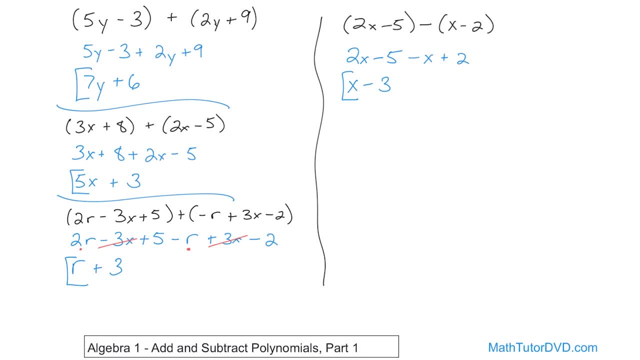 sign so that you can add everything together. all right, so this will be our final lesson, or our final question in this lesson. what if we had five x minus three, t minus seven, and we're subtracting from that x minus two, t minus three. all right, so now we have the same sort of thing you have. 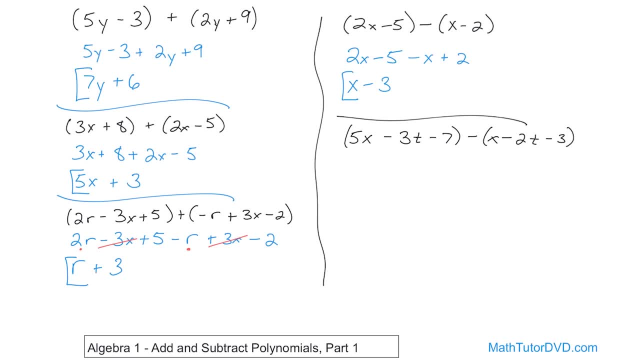 two variables, an x and a t, and then of course nothing here and you're subtracting from it another trinomial, also with x's, t's and constants. so you need to really write everything down and distribute that negative in there. so you're going to have five x minus three t. we're just dropping. 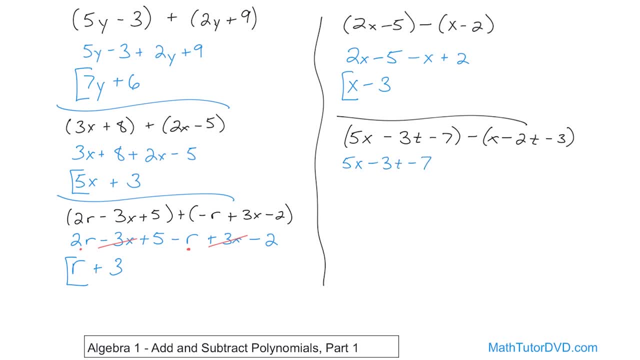 the parentheses here, because there's nothing else we can do inside. we can't actually add those things together and we distribute this negative one, that's going to make that negative x, and then, when you distribute to the negative times, negative is going to give you positive two t, and then what same thing is going to happen here. 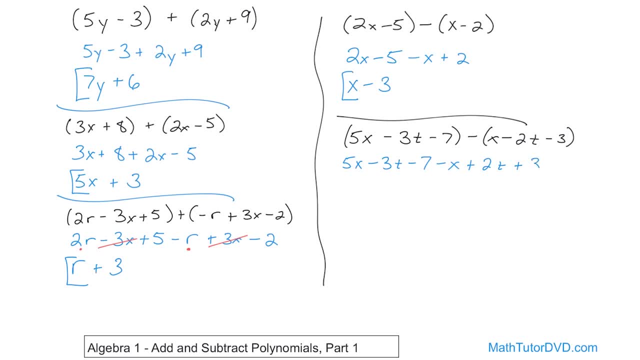 negative times. negative three is going to give you positive three. so now we can start hunting for like terms. we have a five x and we have a minus x. so this is five minus one, which is going to give you four x, and i'm going to go and put a dot under this and under this to remind myself that i've